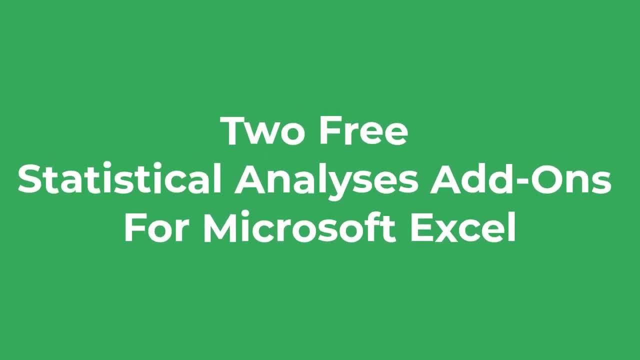 In this short video, I'm going to show you two completely free Microsoft Excel add-ons that enable you to perform statistical analyses on data. So, without further ado, let's get started. The first add-on I'd like to mention is the Analysis Tool Pack. 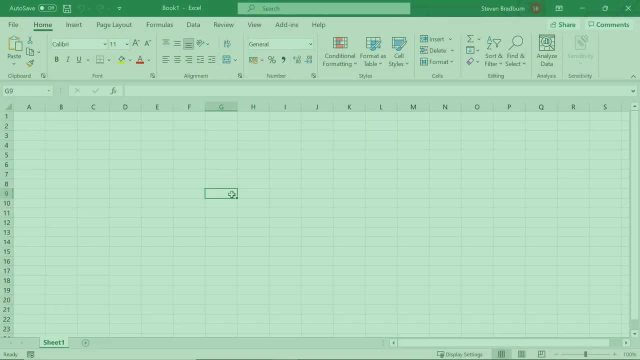 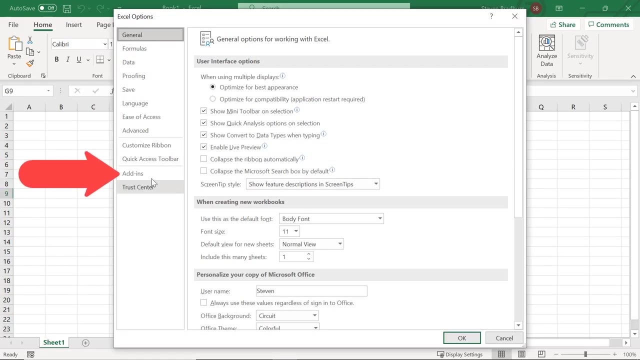 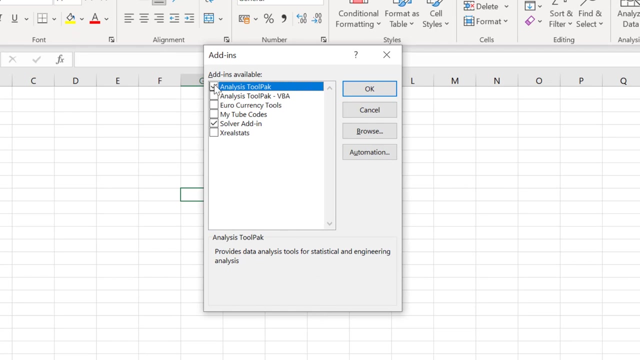 which is created by the guys at Microsoft. To load the add-on in Excel, go to File Options. Then go to the Add-ins tab At the bottom. you want to manage the Excel add-ins and click Go. Then ensure you tick the option for the Analysis Tool Pack and click OK. 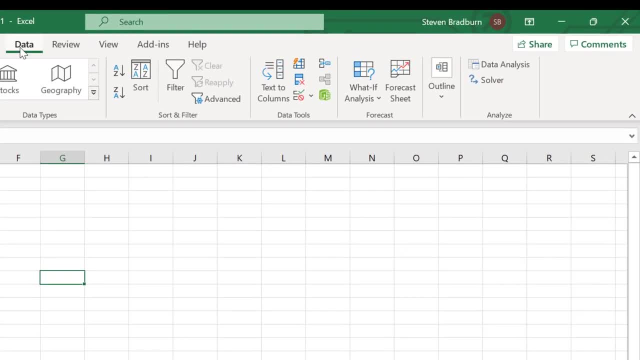 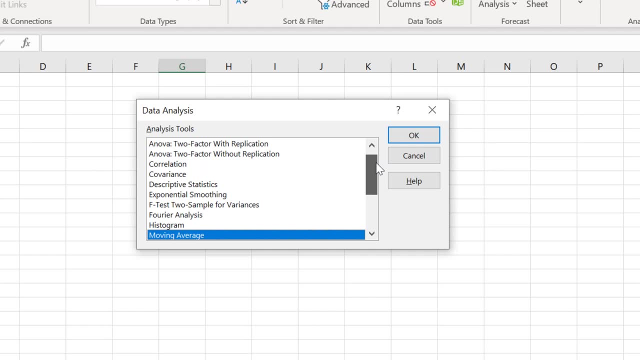 Now when you go to the Data ribbon you should see a Data Analysis button. With the Analysis Tool Pack add-on you can perform a bunch of analyses, including one-way and two-way and over correlation, F and T tests and even a linear regression. I've actually covered. 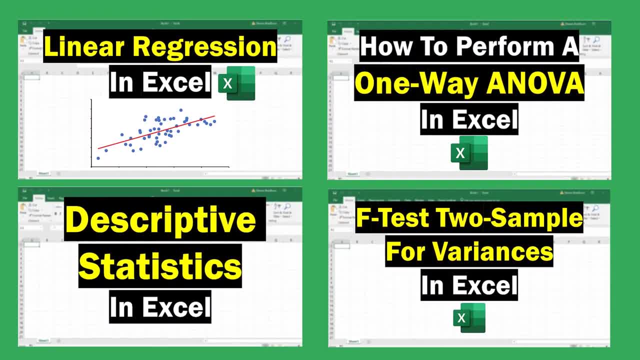 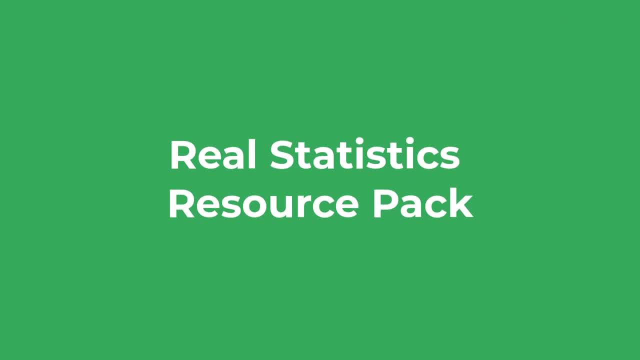 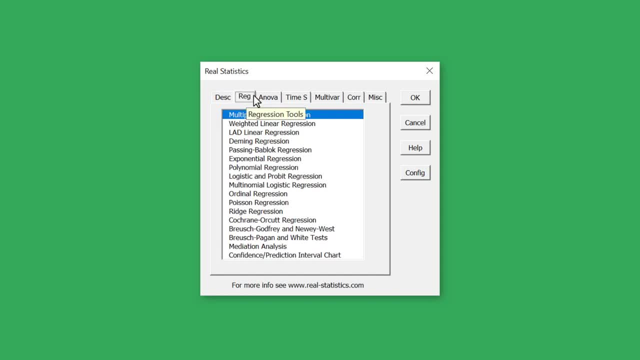 many of these tests in separate tutorials, so be sure to check them out if they interest you. Now, moving on to the second add-in, which is the Real Statistics Resource Pack Created by Dr Charles Zayance. the Real Statistics Resource Pack is an absolutely fantastic Excel. 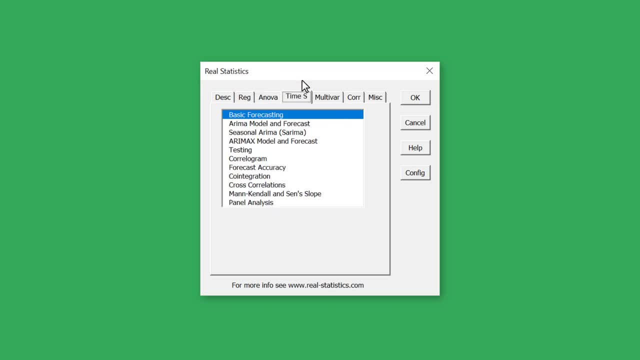 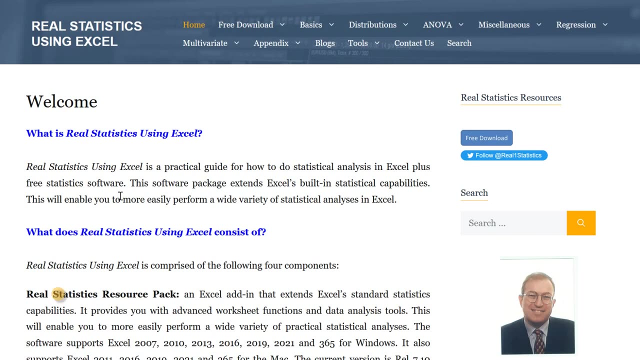 add-on which lets you perform more advanced statistical analyses that you would otherwise expect from software such as SPSS and GraphPad Prism. To install the Real Statistics Resource Pack, you need to head on over to the Real Statistics website and I'll leave a link to it in the description. 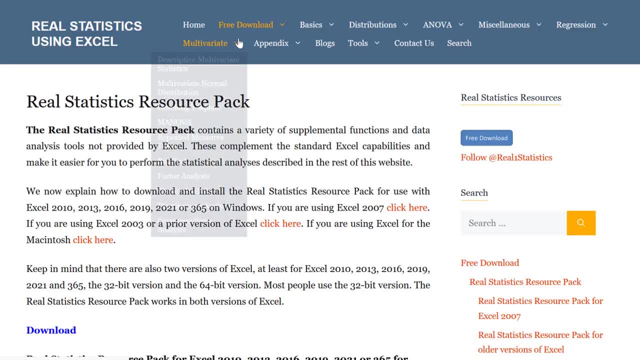 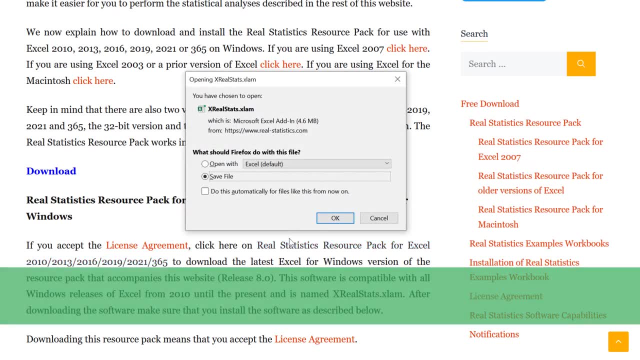 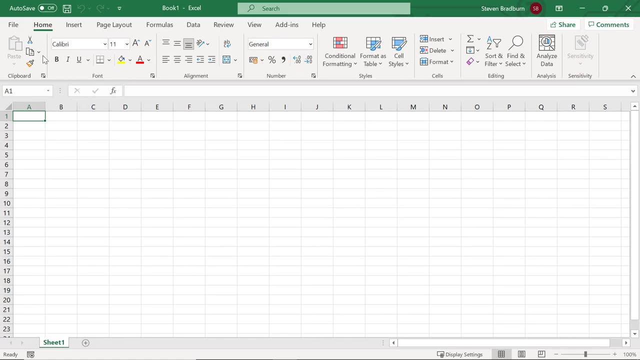 You then need to download the appropriate version of the add-on that is compatible with the version of Excel that you are using. It is recommended to save the file in the following directory: To install the Real Statistics Resource Pack, again go to File Options. then go to the Add-ins tab. 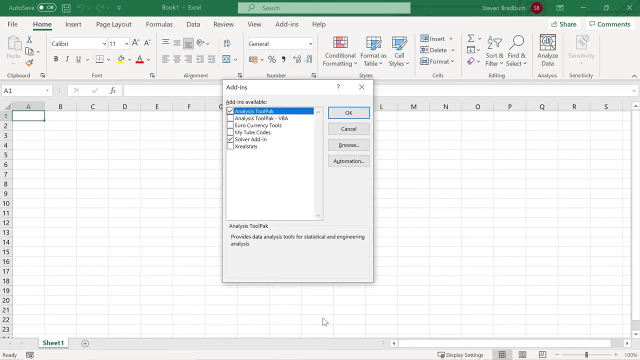 At the bottom. you want to manage the Excel add-ins and click Go. Firstly, ensure you tick the option for the Standard Add-in, then click OK. Then go to the Add-ins tab At the bottom. you want to manage the Excel add-ins and click Go. Firstly, ensure you tick the option for the Standard Add-in, then click OK. 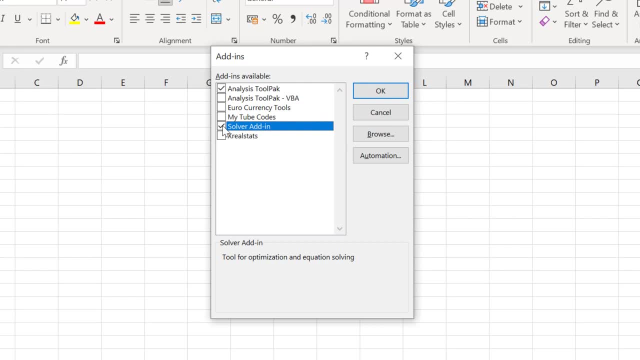 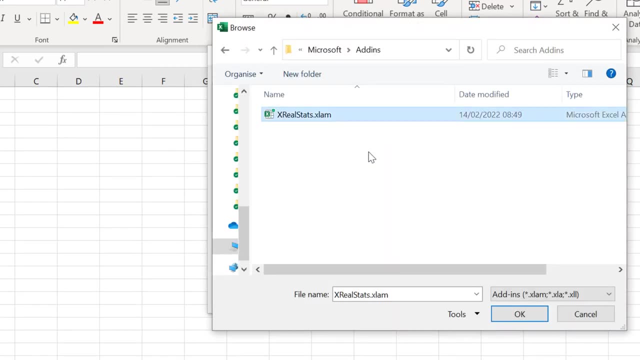 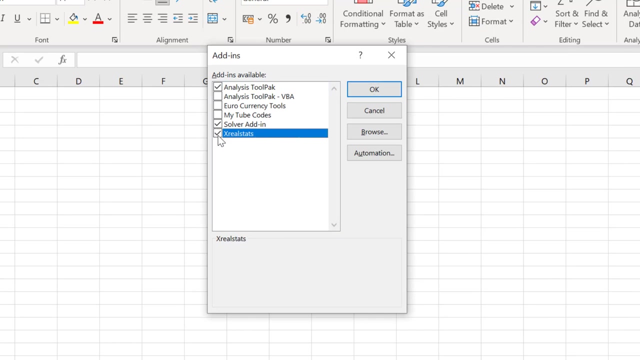 solver add-in, as this is required to use the real statistics resource pack. then, to install the add-on, select the browse button and find the file you recently downloaded. then click ok. ensure that the x real stats option is also checked as this is the add-in, and then click the ok button to use the.